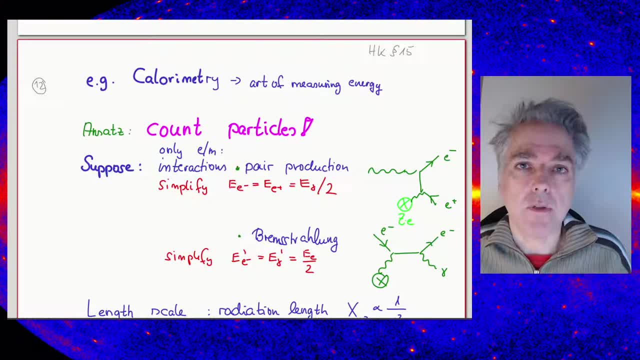 So in this part of the lecture we will talk about measuring energy, And this device is called a calorimeter. It is based upon counting particles, So the idea here is that when a particle enters a calorimeter it produces secondary particles. A shower will develop a cascade And the secondary particles in turn, at least the 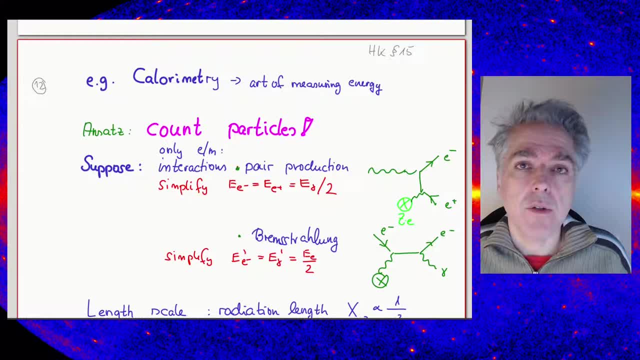 charged particles. they will be registered through a so-called scintillator, which you heard already about in the first lectures, and will be turned into light. So the ionization losses will be turned into light that you can detect with a device and with that measurement. 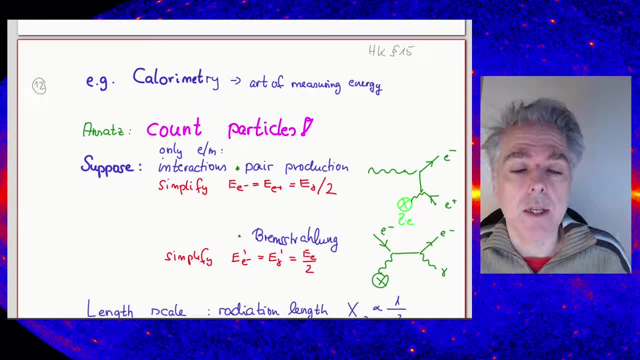 of the light. you basically register a particle. Now, by counting particles, you basically can measure the energy. but how does it work? Now let's talk about a very simple kind of cascade, that is, a pure electromagnetic cascade. In that case we have 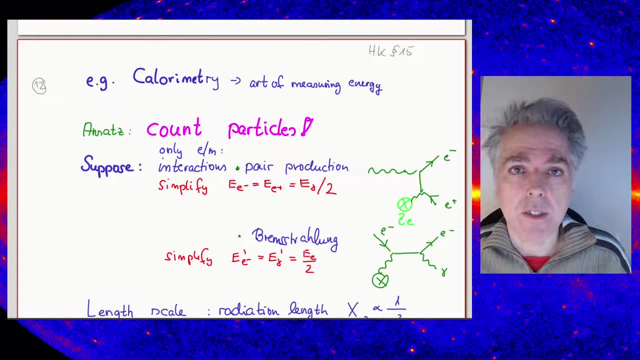 for example, either an electron or a photon passing through the detector and at sufficiently high energies, photon interaction will be dominated by pair production. At low energies you have compound scattering and you have also photoionization, but at sufficiently high energies, basically we would produce mostly only pairs, electron-positron pairs, And for the 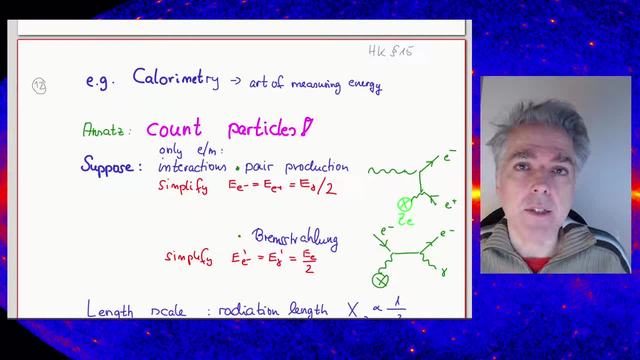 electrons and the positrons. you have two competing energy loss mechanisms. One would be ionization losses, and these dominate at low energies, At high energies, above a so-called critical energy. the energy will be mainly lost through bremsstrahlung. So bremsstrahlung is a process. 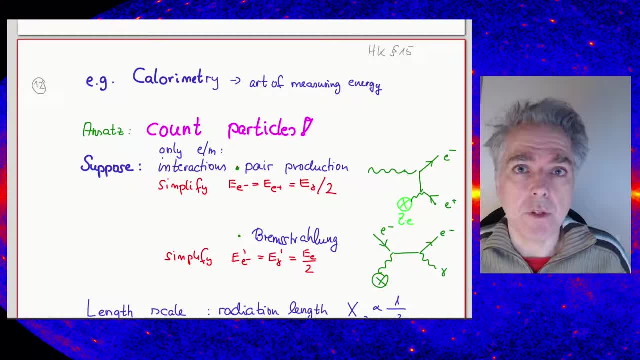 in which the electron is deflected by the Coulomb field of the nucleus and because of, classically speaking, the acceleration it starts radiating. In the treatment of quantum field theory, this is an emission of a single or multiple photons, given that it basically. 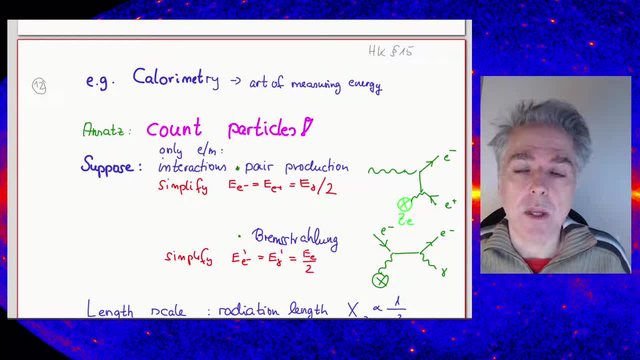 couples to the virtual photon of the nucleus. Both interactions, that is, pair production and bremsstrahlung, share some common features. One of the things which we will simplify for now is that the energy of the incoming particle is shared between the outgoing particles For the 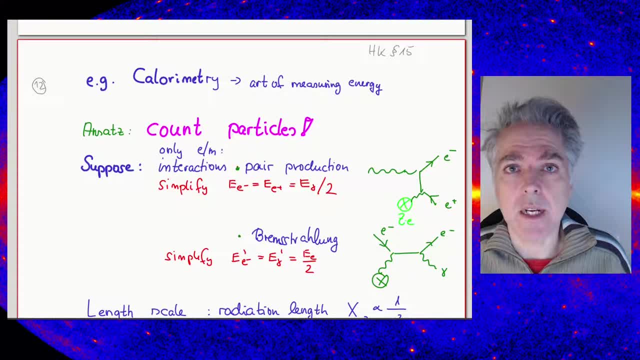 pair production, that's electron and positron. The energy of the incoming particle is shared between the outgoing particles. For the pair production, that's electron and positron. For the pair production, that's electron and positron. And for bremsstrahlung, that's an electron and a photon. 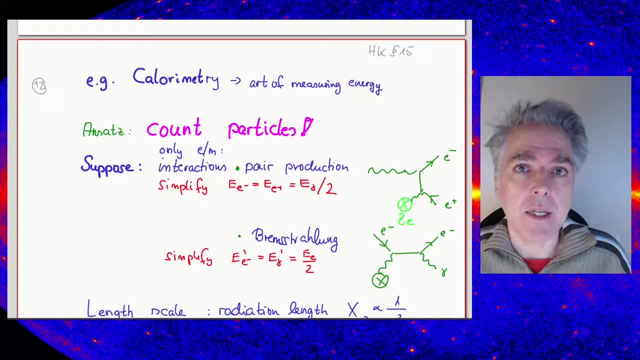 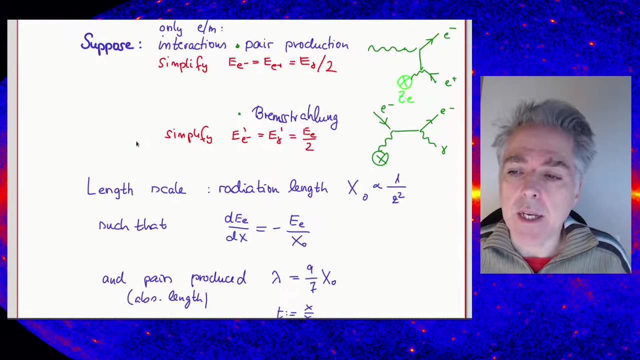 And in the most simple approach that we want to use here to get an idea on the mechanism, we just assume it's shared in equal way. In detail this is a bit more complicated, but this is, on average, not a bad estimate. So the length scale over which particles interact in the medium is characterized. 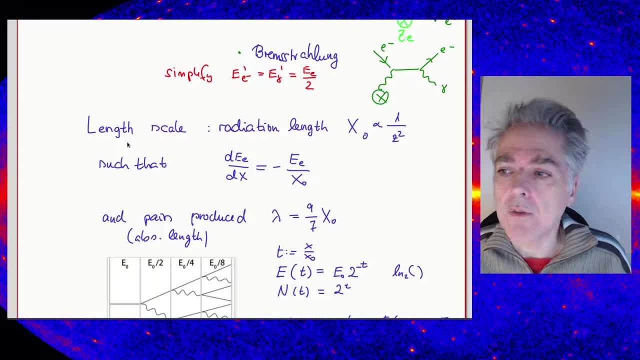 for the bremsstrahlung by something we call the radiation length. So the radiation length x0, called, is proportional to one over charge number, z squared of the medium in which the electron propagates, And the radiation length characterizes the energy loss. So if you look at, 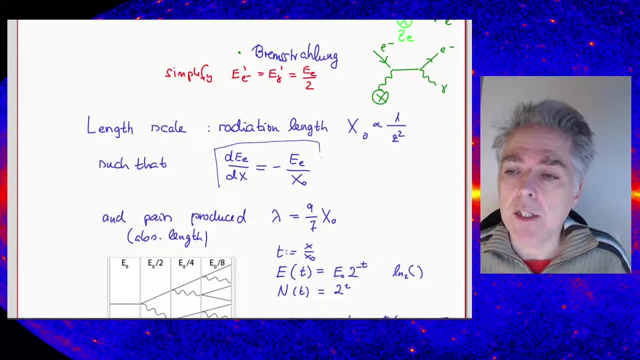 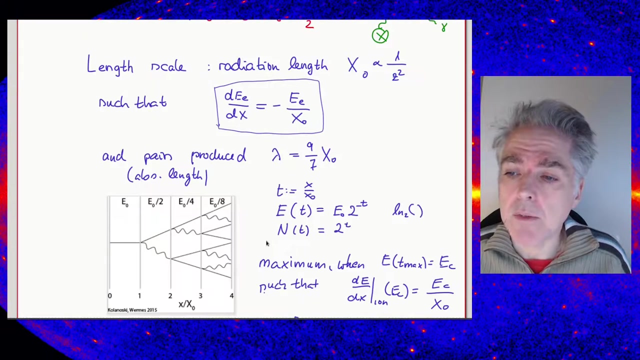 that equation. here you see that energy is lost over a distance which is the radiation length For pair production. photon will basically produce an electron-positron pair, again in the field of the nucleus. I have shown here the two Feynman diagrams for pair production and for bremsstrahlung process And the distance over. 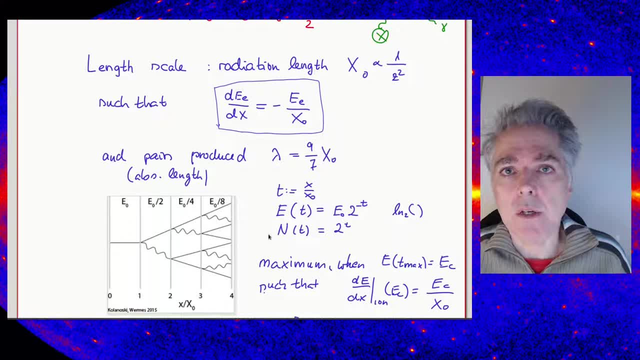 which a photon on average is being absorbed is relating to the bremsstrahlung radiation length. More accurately, it's nine seventh of a radiation length. So we can make a very simplifying assumption now. we'll say that basically, after roughly one radiation length, electrons will bremsstrahle and the photon will pair produce. 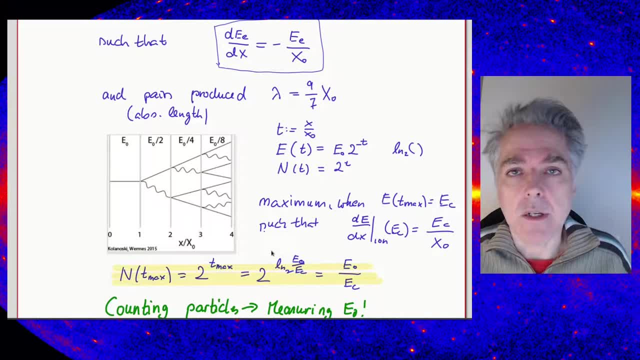 So in this way we can make a very simple schematic diagram which shows us how particles will behave after a number of radiation links. So we introduce this quantity, t. T is defined as the ratio of path length over radiation length. so t counts the number of radiation links on the medium And in the very simplified scheme that we say particles. 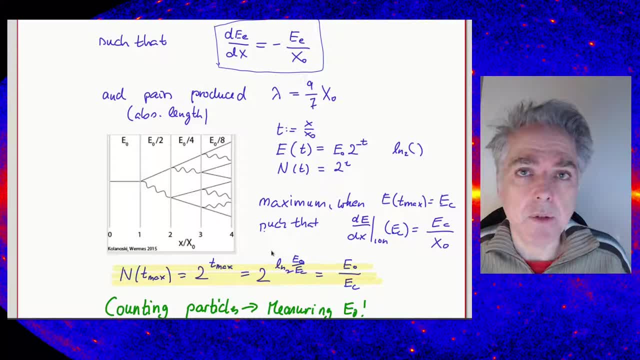 when they pair-produce or do Bremsstrahlung. they basically produce secondary particles which will have each half of the incoming energy We can end basically the particles will pair-produce and do Bremsstrahlung after around radiation length. We can divide the medium into. 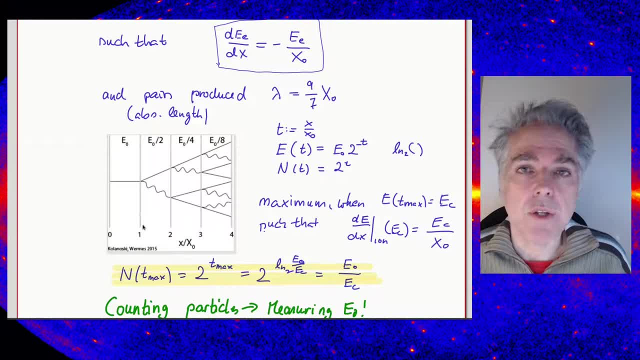 in this case four radiation lengths. So after the first radiation length, the incoming- in this case electron with energy E0, goes into an electron and a photon, which each have E0 half. After two radiation lengths then we will have E0 quarter. 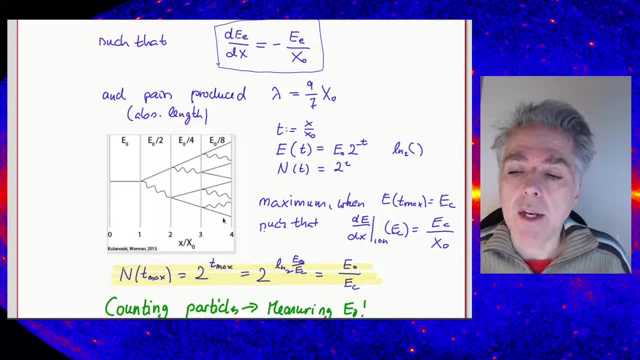 shared by three electrons and one photon. And after the third or after three radiation lengths, we will have an average energy of E0- eighth. And this will be shared by three photons and one, two, three, four, five electrons. Now turning that into equations: 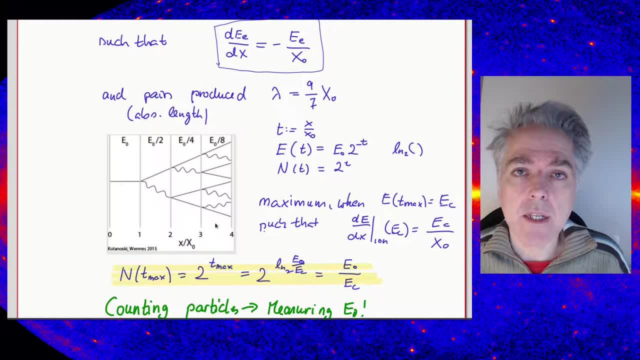 we could basically state that the average energy after T radiation length is given by E0 times two to the minus T, And the number of particles after T radiation lengths will be, on average two to the power of T. So the maximum of this process will, however, be reached. 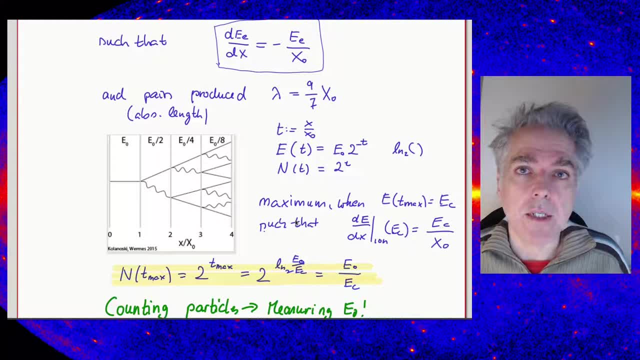 once the energy or the average energy of the particles hit either first the pair-production threshold or they hit the energy below which ionization losses start to dominate. It's usually the critical energy which is hit first, because that's larger than most media. This is larger than the energy. 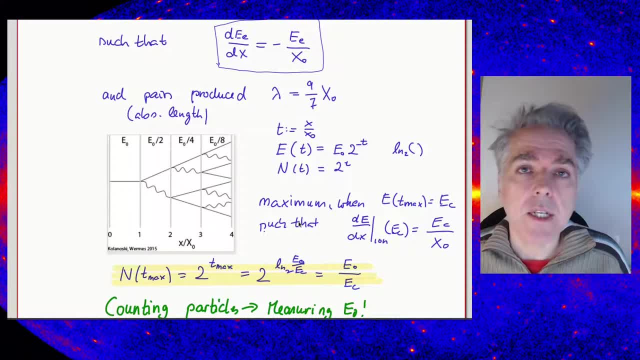 the average energy for pair-production. So this critical energy is the one which determines the position where the maximum is reached. Because once the average energy falls below this critical energy, the electrons will not do Bremsstrahlung anymore, but they will predominantly do ionization losses. 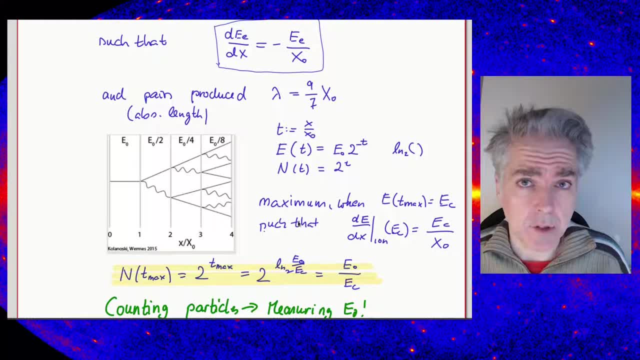 and they will be just lost. Keep in mind, the electrons always do ionization losses. It's just that one energy loss channel dominates over the other, And so we define that the critical energy is, given that the energies that are lost between ionization. 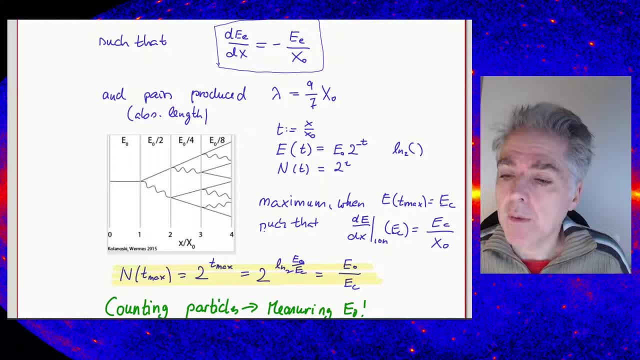 is equal to the energy lost in Bremsstrahlung, And then we can basically take this first equation here, that is the energy, and we take the logarithm to the base of two if we want, And then basically we get a very simple equation. 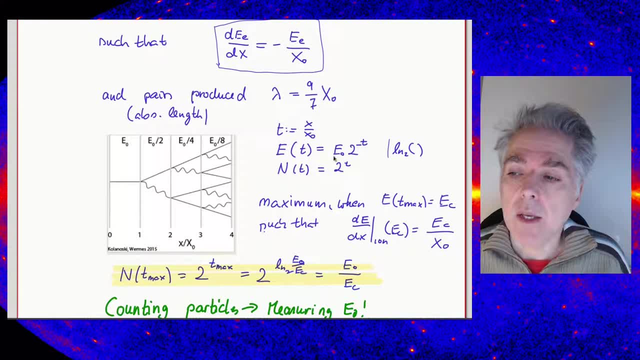 which says that the maximum energy, that is- we'd look at this equation- when the maximum is reached, so E at T max. So the average energy will be then E-critical, and on the right we have zero times two to the minus T max. 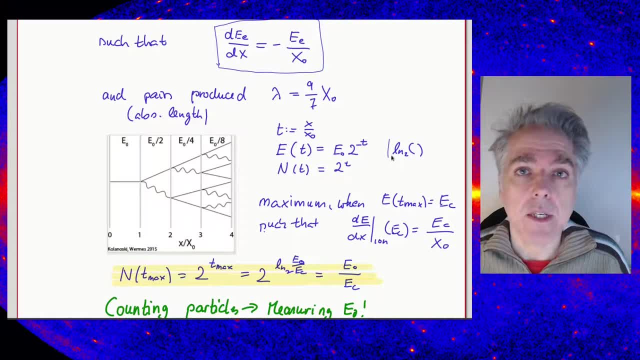 and then we take the logarithm And then we'll have T max is given by the logarithm of two of E zero over E C. So this will be depending upon the energy, but only logarithmically, And the number of particles in the maximum. 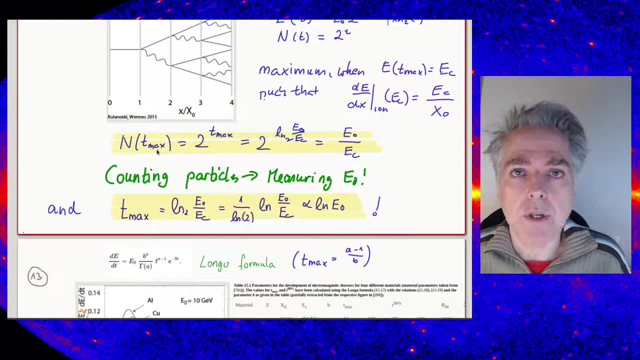 we basically get when we put in the number of radiation lengths which have been passed until the maximum is reached. So this gives you two to the power of T max, And T max, as we saw now before, is logarithm two of E zero over E C. 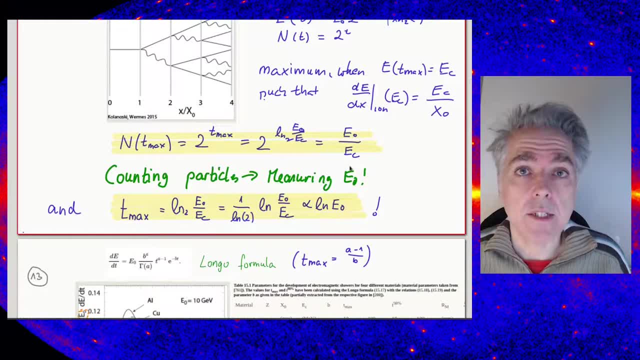 So, then, the maximum number of particles scales directly with the energy of the incoming particle divided by something which is just a constant of the medium in which we're dealing with. So once we're able to count the number of particles, for example the maximum, 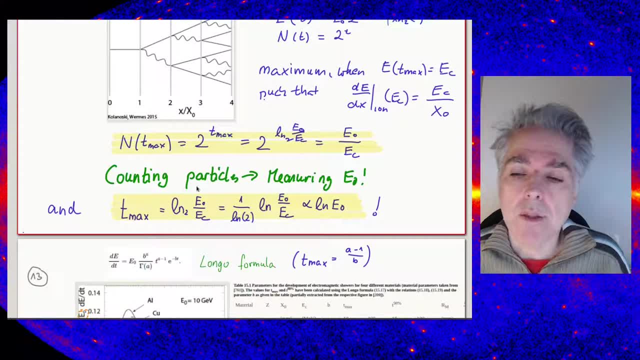 we basically measure the maximum energy. The maximum position itself depends also on the energy. So in principle also measuring the position of the maximum gives us a way of of estimating the energy, but it depends only logarithmically on the incoming energy. 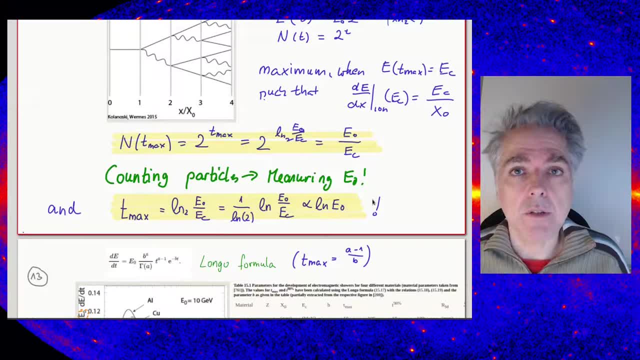 So this is something which has to be taken into account, So that, for example, a calorimeter has to be sufficiently thick in terms of radiation links to still capture the maximum, And it has to go, let's say, roughly eight to 16 radiation lengths beyond the maximum. 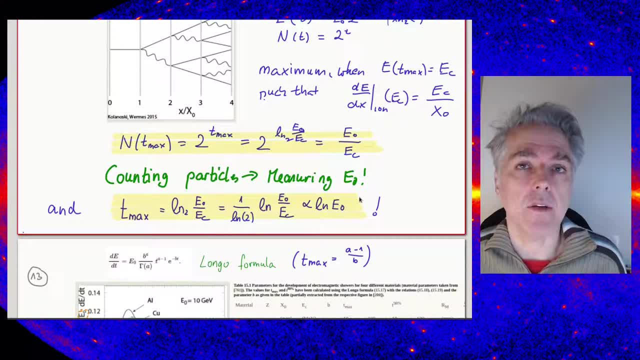 to really capture, let's say, 98% of the energy or the particles which travel through this calorimeter. So this is something which we have to take into account when we built a calorimeter: It always has some limitation when it comes to increasing energy. 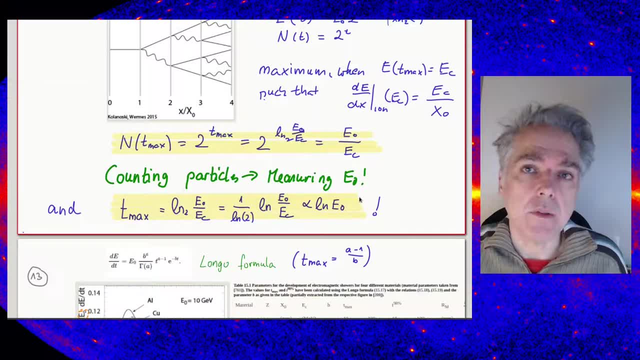 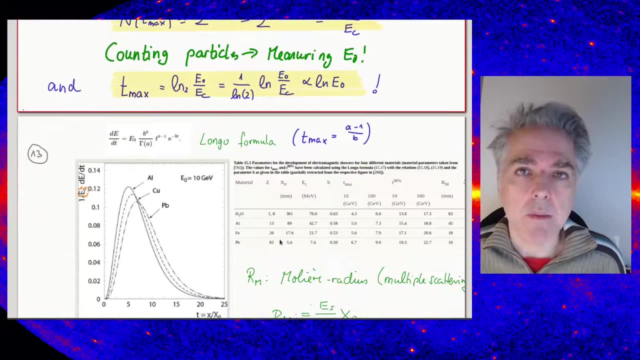 because at some point the show maximum would basically lead to a leakage of the particles out of the calorimeter. We will not be measuring all the energy anymore. We can look at this a little bit in more detail. There's various ways of parametrizing. 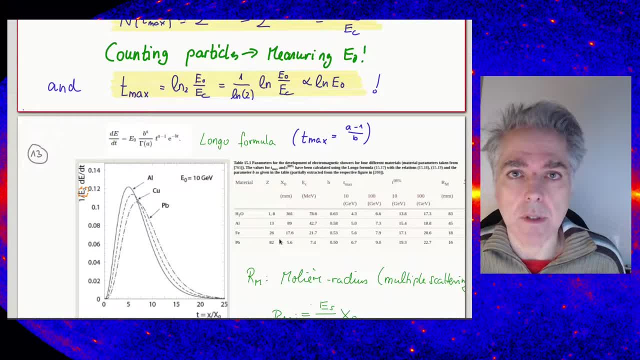 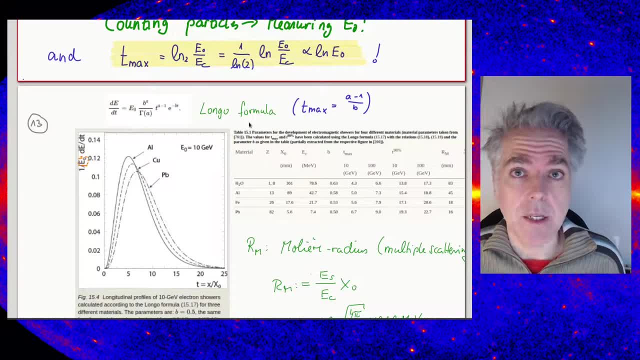 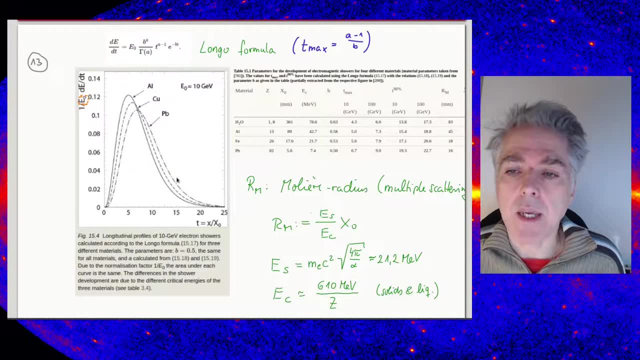 which I just flashed you briefly, the so-called Longo formula, which I just flashed you briefly, the so-called Longo formula, which tells us how much energy is dissipated as a function of shower depth. And you see that, for example, here, 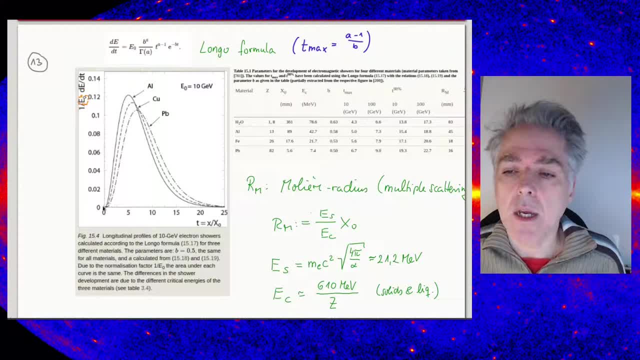 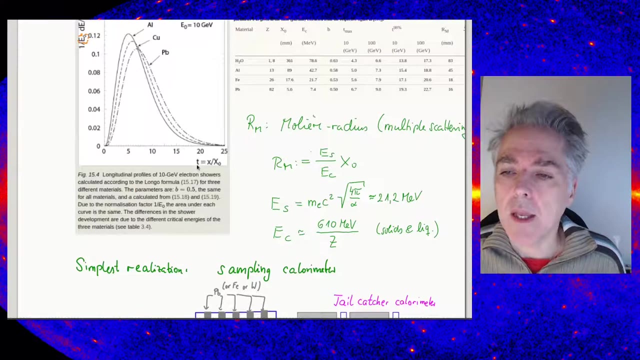 you see the energy deposited in a shower as a function of the entrance, And there you see, there's some slight differences between the different medium that you choose, And this is basically captured by some parameters that you can use in the Longo formula, Besides the longitudinal development. 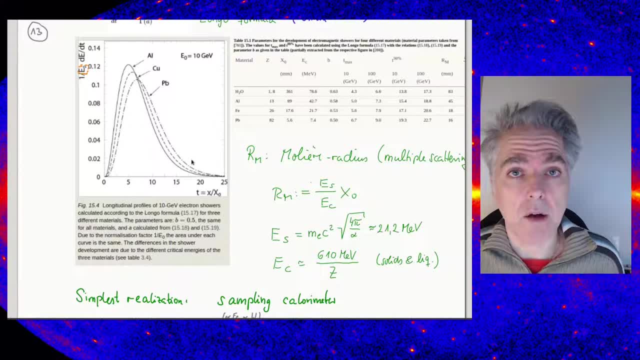 you can also look at how broad the shower is transversely to the direction of the incoming particle. That's the so-called lateral shower development. And the most important quantity here for a pure electromagnetic shower is the so-called Moliere radius. The Moliere radius is the radius. 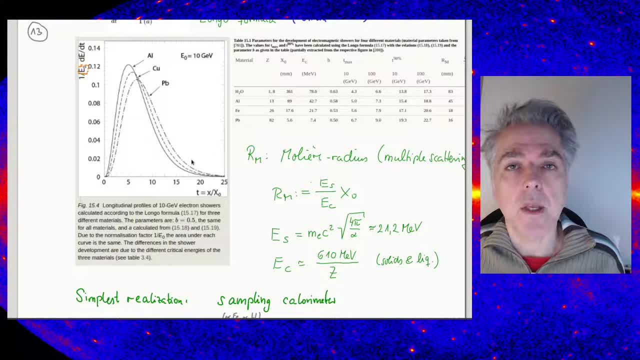 in which the particles will be confined laterally. The Moliere radius has to do with the multiple scattering, So electrons- electrons on the way through the medium- will be scattered by passing close to a nucleus and see the Coulomb field of the nucleus. 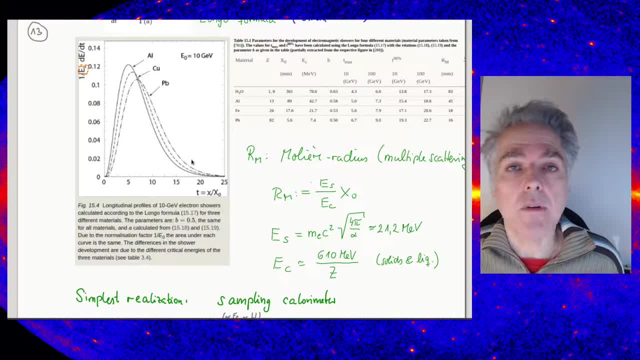 And this is a stochastic process, And the Moliere radius basically gives us a measure of how, broadly speaking, the shower develops laterally, And it's given by its proportion to the radiation length, x0.. And it's also depending upon something which is called ES. 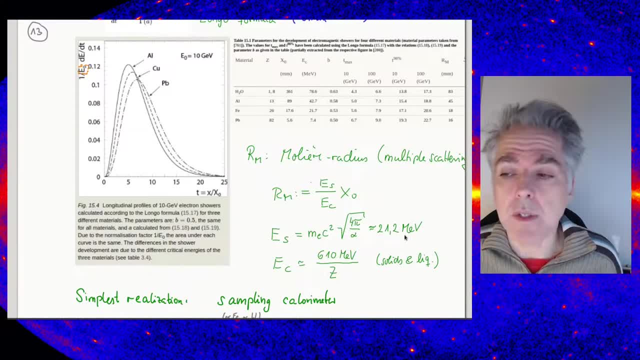 This is the scattering energy, which is a natural constant. So this is medium independent. What do you want? 0.2 MeV And the ratio of ES over EC, where EC is already introduced. critical energy, where I give a very simple parameterization, which. 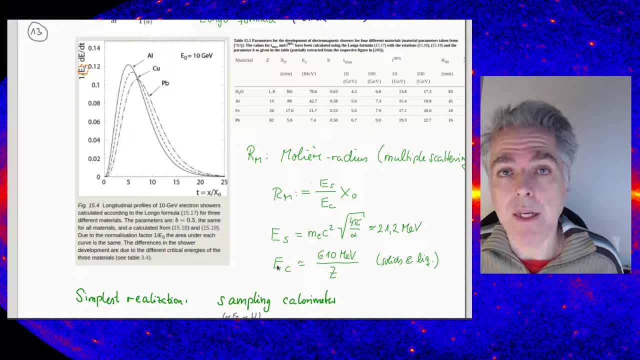 is sort of useful for estimating the critical energy And it depends upon 1 over z, so the charge number of the medium. So it goes with 610 MeV roughly over z, And so the Moliere radius is given up in this table. 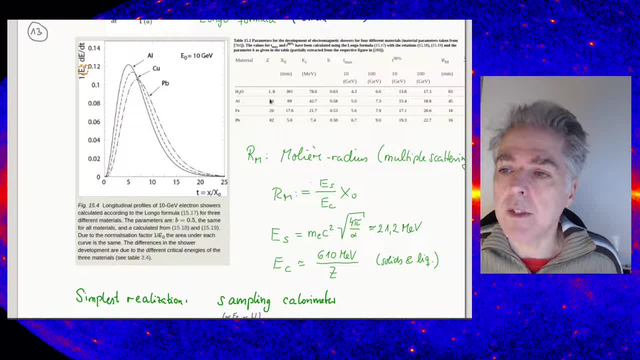 So you see, this is now And distance in units of millimeters And you see, for example, the Moliere radius for lead is something like 1.6 centimeters And for aluminum it's something like close to 5 centimeters. 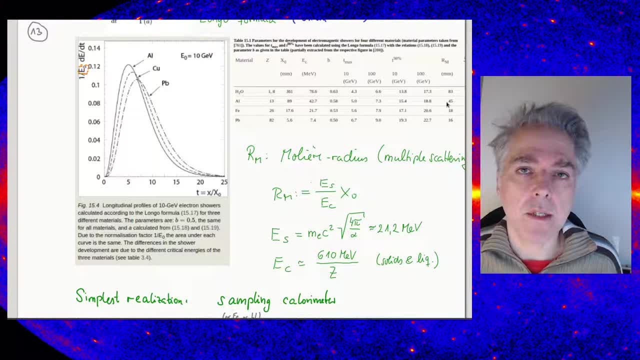 Now, the Moliere radius is something, therefore, which, if we want to design a colorimeter and we want to capture it, it makes sense to sort of make the size of each particle detection unit about the size of a Moliere radius. 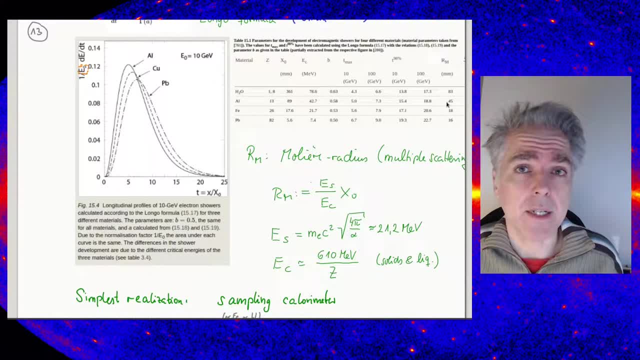 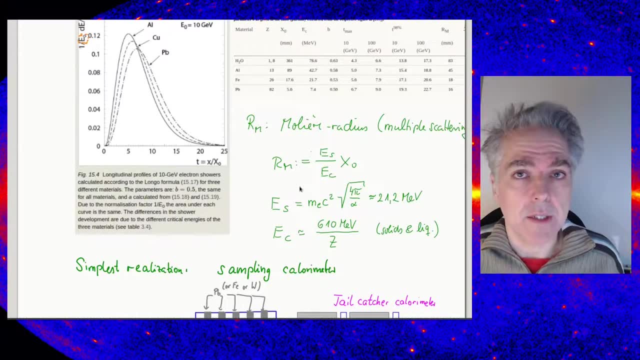 because this is basically where we can measure then the shower, The shower particles, And they're confined in that radius And it doesn't really make sense to make it much smaller than that in a single segment of a colorimeter, because we would basically oversample the shower. 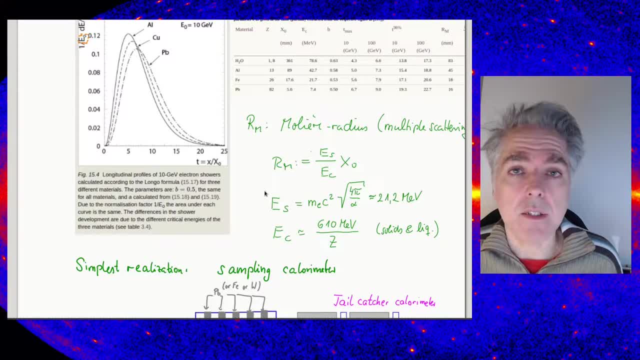 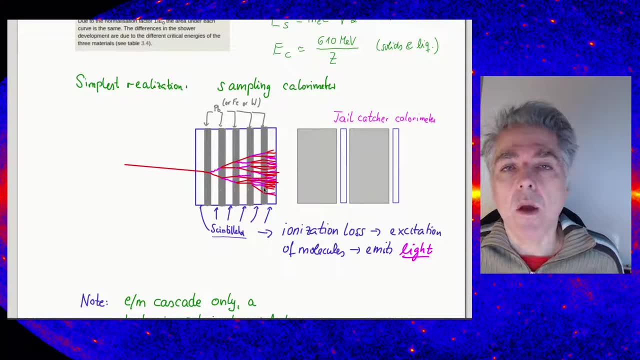 development, And that would be basically a waste of channels and of detector complexity. Now, the simplest realization would be to produce a setup where we detect all the particles passing through in one way or the other And we would count them and therefore determine the energy. 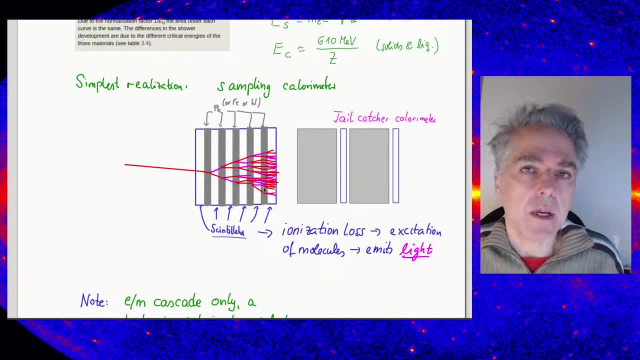 In the more realistic case that you do not want to build a detector which is fully sensitive, that would be made of, for example, a scintillating material. you would interleave layers of conversion material with a large surcharge number, where the Bremsstrahlung process. 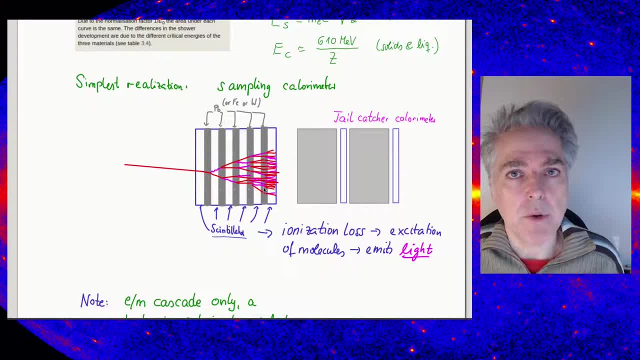 takes place And this would make also the colorimeter more compact, because typically the detection of light happens in, for example, organic scintillators- And we'll come to that, We'll talk about that in a moment- And that means these are very lightweight, small surcharge. 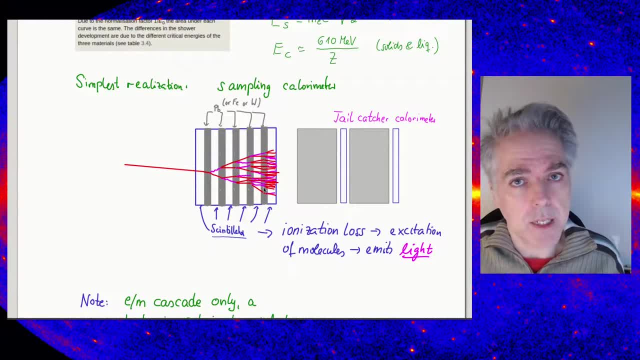 number, And so this thing would become very, very big. So by putting lead layers, for example, in between, we separate the detection and the conversion, And this is the so-called sampling colorimeter, And such a building block would have about the size. 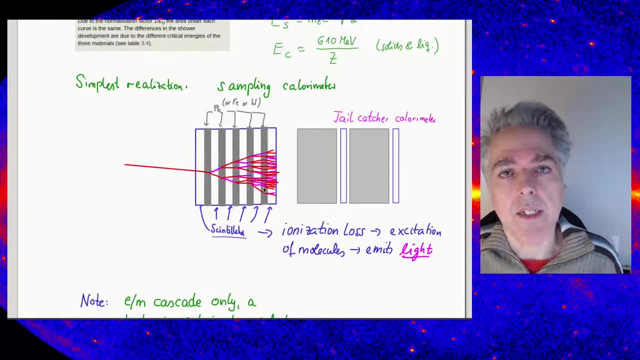 of a Moliere radius And it would consist out of layers of scintillating materials and, for example, layers of lead which would be sort of the size of about a radiation length, so about half a centimeter of lead. 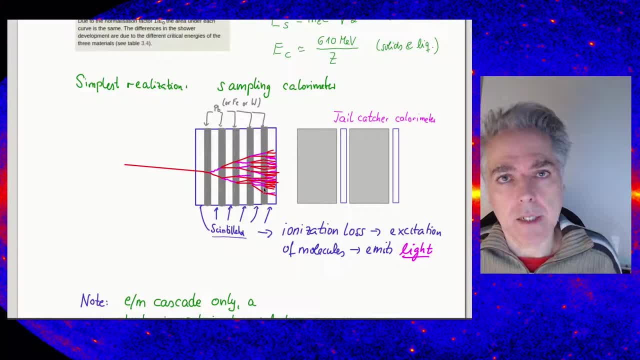 And then we would measure the passage of the charged particles in the scintillator. The amount of light that we register in the scintillator is proportional to the number of particles, And therefore we would count the number of particles and reconstruct the energy. 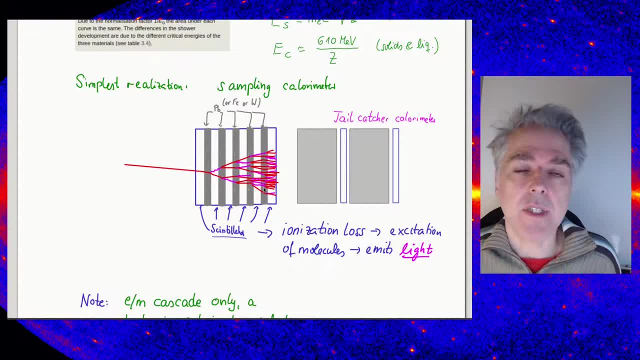 In order to catch also the part which would leak out of the sampling colorimeter, you would complement the colorimeter with a tail catcher colorimeter which consists out of larger blocks of conversion material And then smaller numbers of layers of scintillating material. 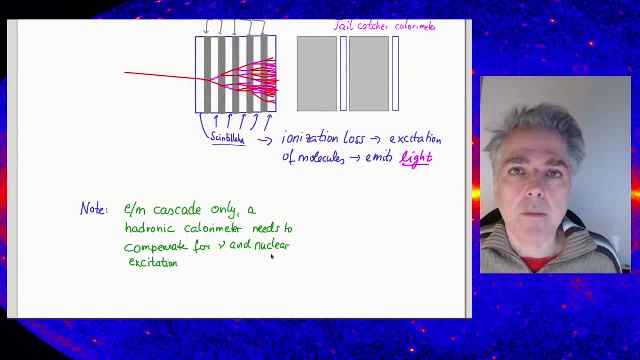 Now just a note which I want to make here before we turn to the scintillator process a little bit. This has all been discussed in the context of a pure electromagnetic cascade. In the case of a hadronic colorimeter, where you want to measure the energy of, for example, 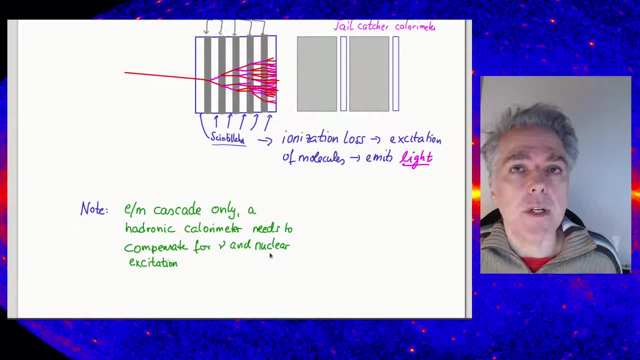 a proton which passes through. there would be a further complexity involved, because the hadrons do not. They will produce only electromagnetic particles, but they also produce, for example, mesons, And mesons will decay. They produce muons, They will also produce neutrinos. 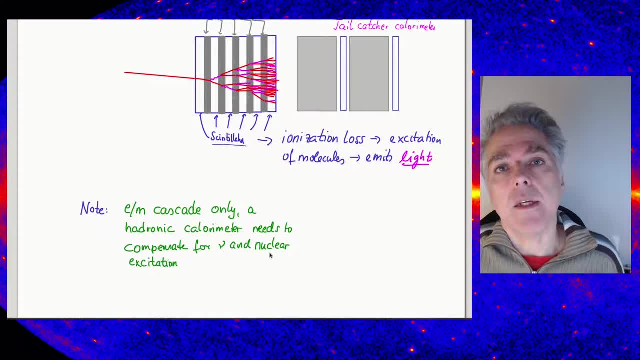 And so, therefore, some energy will basically pass through and we will not be able to register it. So a muon, for example, will just basically make ionization losses, but it will be counted as one particle. So this would not be in the spirit. 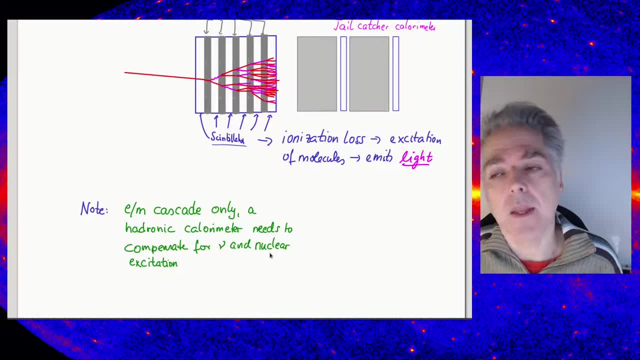 of measuring the energy by counting secondary particles in the cascade, And so another process is that Hadronic or strongly interacting particles will also lead to excitation of the material, which would make the situation a bit more complicated, But however, the whole idea is still the same. 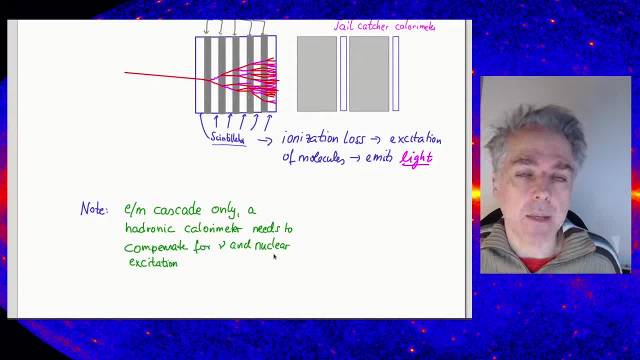 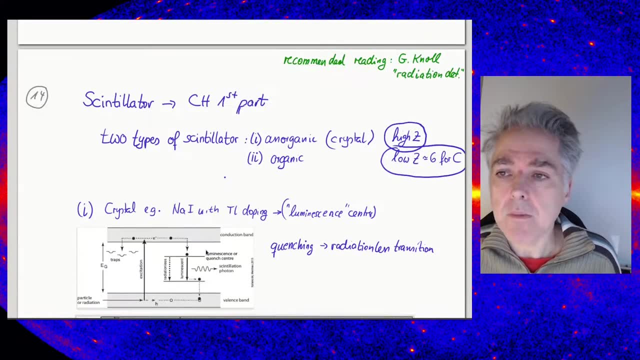 You will still measure number of particles and then find a way, for example, capturing the muons or calibrating carefully the losses which are going invisible. Now let's talk for a little while about the way that the scintillator works. There was, of course, some mentioning of scintillators. 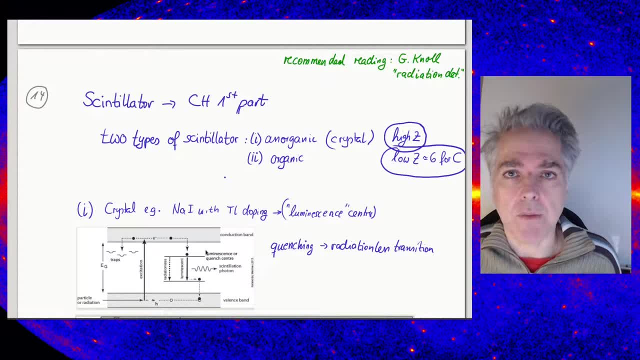 in the first part, But let me just briefly go through some of the things which are relevant for scintillators to make sure you understand what kind of materials are typically in use and what differences there are. Now there's, roughly speaking, two types of scintillators. 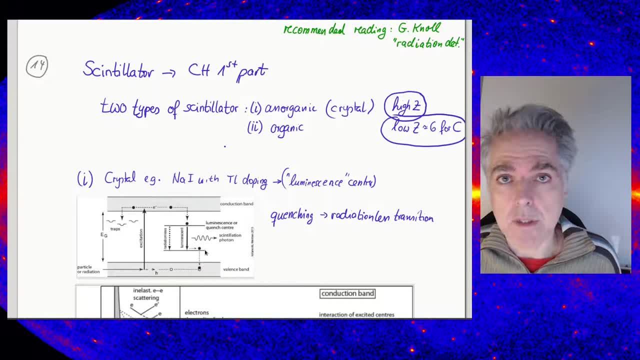 And there's so-called anorganic or crystal-type scintillators and organic scintillators. So the main difference to capture in essence is that the anorganic scintillators- they are usually made out of a material which are large. 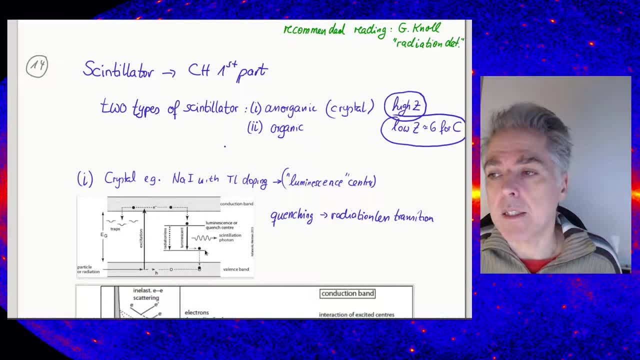 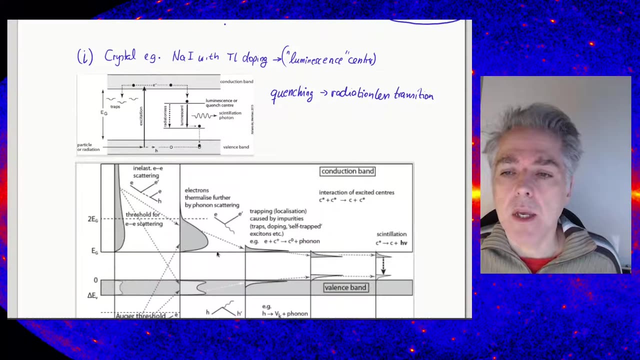 which has a large charge number, is more solid, more massive, Whereas the organic ones are made out of molecules which are carbon-based and therefore they have a charge number of six. Let's talk briefly about the light production process in an anorganic scintillator. 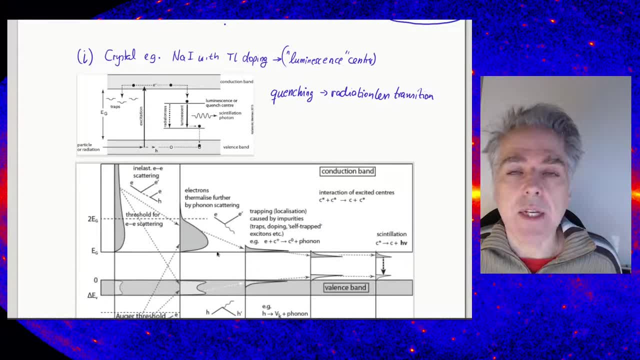 So a crystal, as an isolator, consists out of a valence and a conduction band, And once a particle passes through and ionization losses are being deposited in a crystal. you have various ways of exciting the crystal. Essentially, you could, for example, excite phononics. 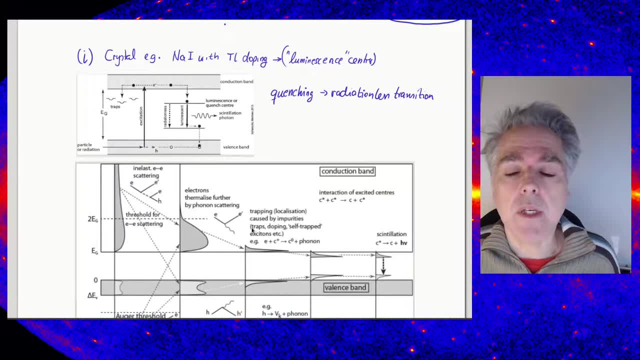 or some acoustic waves, And you could also excite, either directly or through the phonons, electrons And you would lift them up from the valence band into the conduction band. In the conduction band you would then have a freely moving electron. 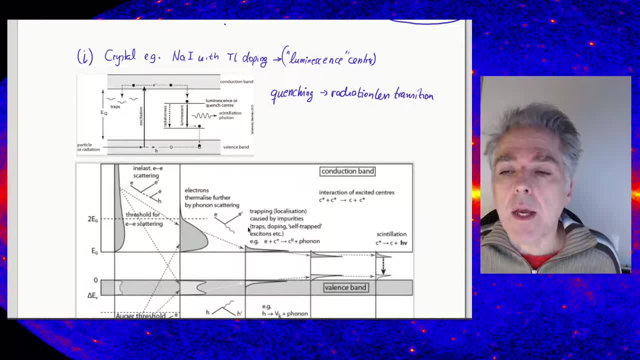 And in the valence band you would have a hole. Now they would ultimately require recombination at some point. But there's two different ways that the recombination can take place. One of them, the electron basically, is getting trapped and it will recombine at a very later stage. 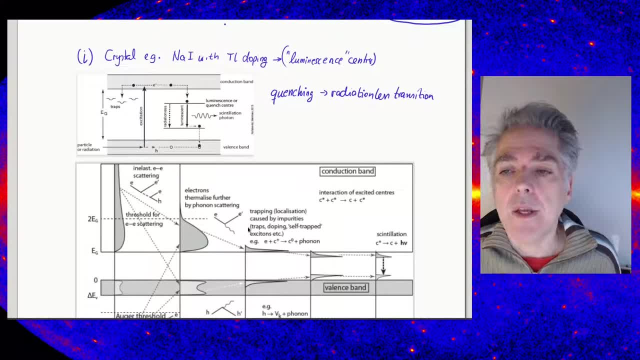 So it takes a long time and it's not of relevance anymore. The other one is that you could have the electron going back to the valence band through either a radiative or non radiative process, The radiative process, as the name says. 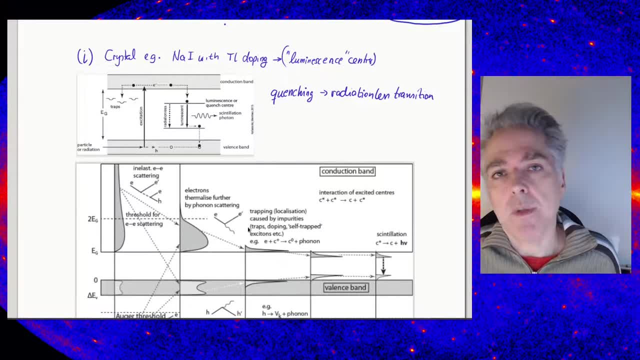 will produce a scintillation photon, And then this will be something that we can register In the radiationless. this is something we call then quenching. The energy would be lost, in a sense that we do not see any visible light coming out. 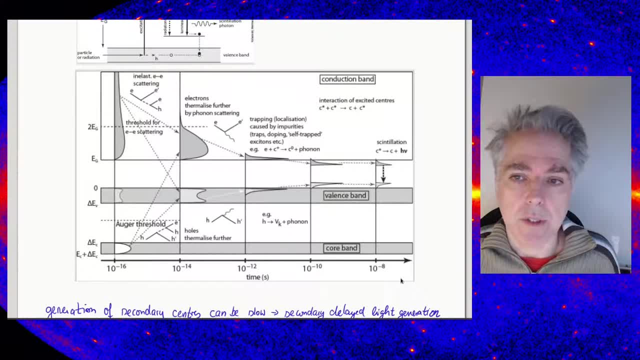 In a little bit more detail. if you look at the time sequence of this happening again down here, you have the valence band and also, in addition to that, the core band, Because the core band is essentially the band of electrons which are very tightly. 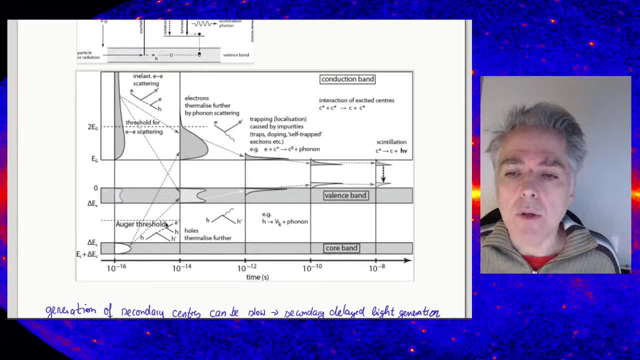 bound to the nucleus. So you would basically say that the electron is going to be released from the core band to the conduction band. So you would basically have, for example, sufficient energy to excite an electron out of the core band up into the conduction band. 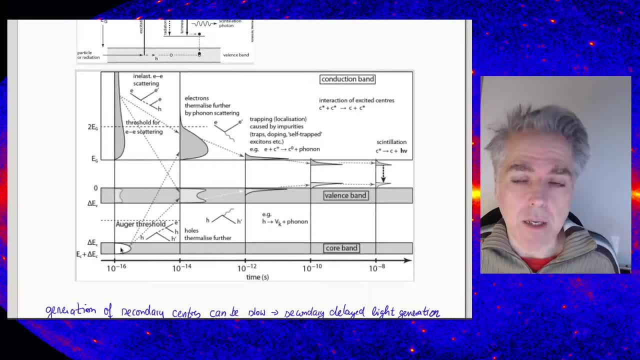 And given that you deposit a lot of energy, we talk about several MeV and the band gap is, let's say, 10 electron volt or more, So the electron will have a distribution of energies or the electrons will have a distribution of energies. 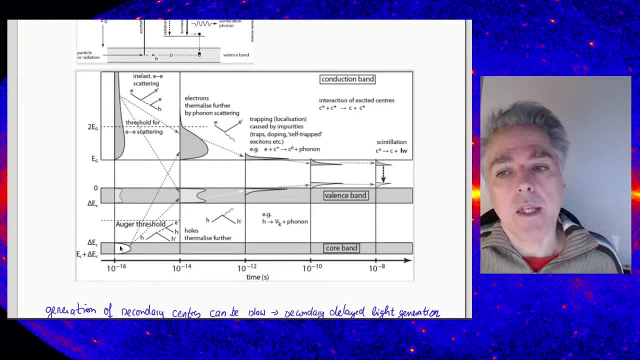 in the conduction band, which is rather broad, And so there is actually some additional process which bring down the energy of the electrons. And these are happening fast, because this is essentially scattering, which takes place on a very short time scale, at the level of 10 to the 4th minus 14,, 10 to the minus 15. 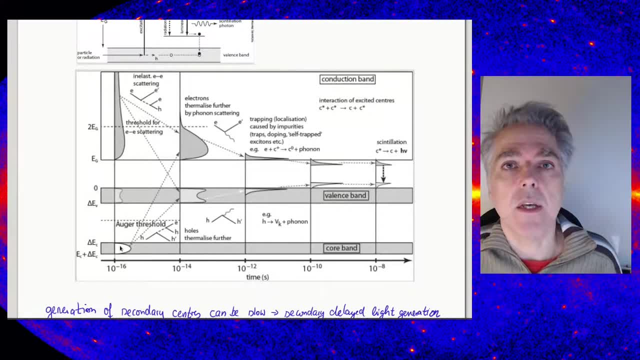 seconds relating to the average mean free path in the conduction band, And so basically this will thermalize and produce in a broad distribution, but it will narrow down further and further and further And at some point you will have then the electron. 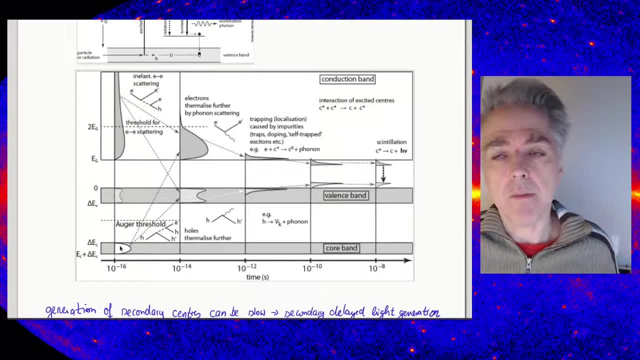 and the hole forming and they can recombine and produce scintillation photon. So this process takes of the order of nanosecond and longer, And that's important to keep in mind. So this process is intrinsically something which can take quite some time because of the way. 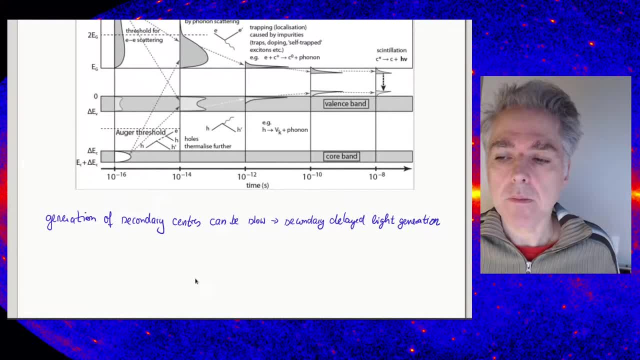 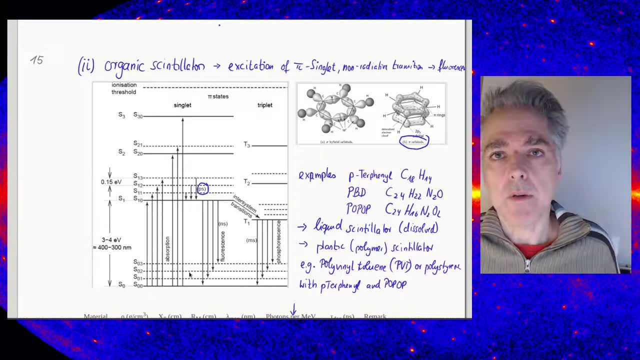 that the electrons thermalize in the system And the organic scintillating material on the other hand, we talk about excitation of energy. So in addition to that there can be also some other kinds of physical opposition that are complicated to understand without any kind. 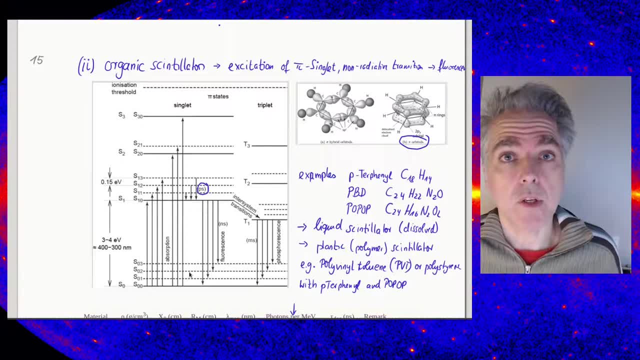 of explanation to what the elements actually shape and generate as well, And this is an example of an initially required пл板 there. in more detail in the causes and concerns cycle as well. This is what this is involved in, So there could be something small, oreki. 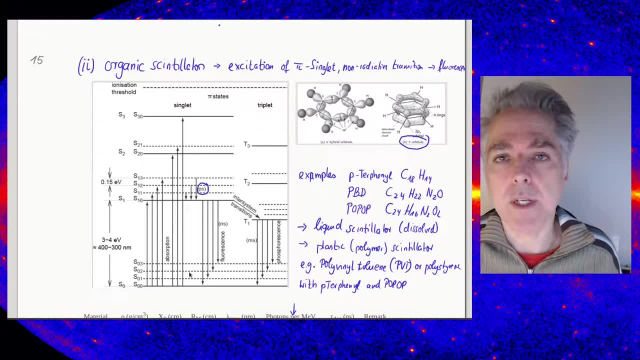 something large or something large. It could be a relative function, Or you could use some sort of model with a fundus, Or we could be working with aндroper orbitals. when you form these kind of aromic rings And then what happens is that you basically 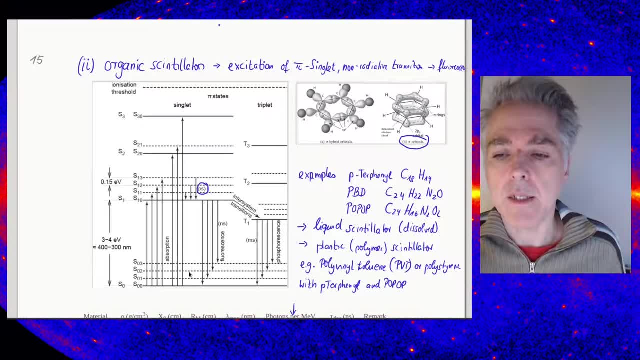 excite a state in this band of pi electrons, It's then de-excited within that band, and this happens very, very quickly until you basically hit the bottom, the lowest state of these kind of bands that are forming. So this takes place only picoseconds and after 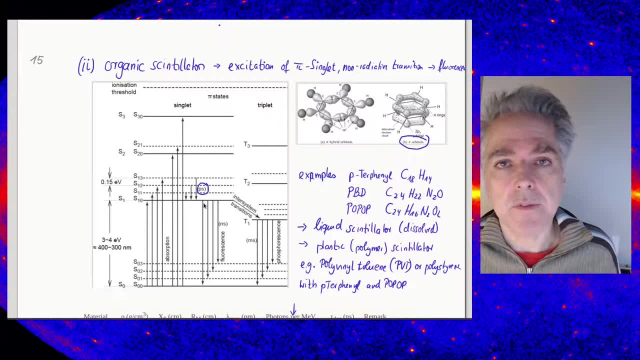 that you will have a fluorescence that is a radiative decay transition going to the base, to the ground state, And that's the one that we want to use. There's also some possibility that it will go into a triplet state, but that basically takes even longer. 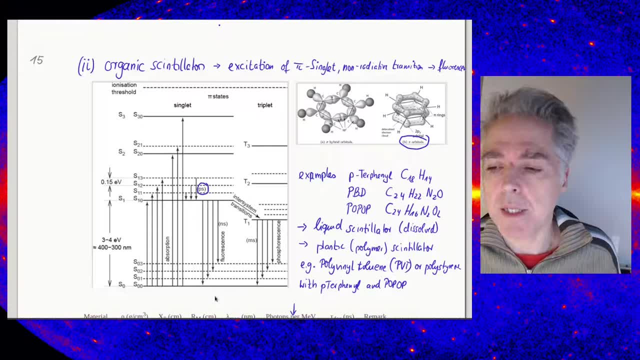 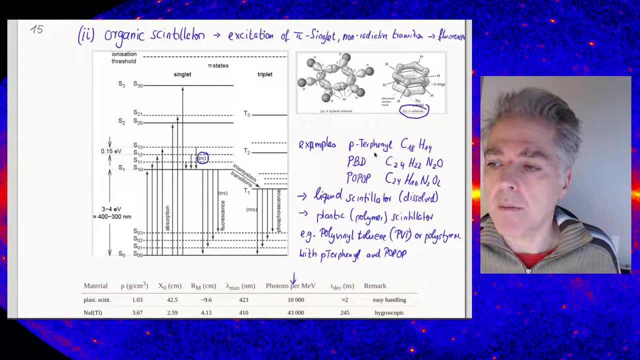 so this would be a very delayed kind of emission, which comes then out after milliseconds because these are the bands that are forming. So these are forbidden interactions, forbidden transitions, And some examples are given here. so p-terphenyl, for example, C18-18-8-14 is a very common molecule which is used as 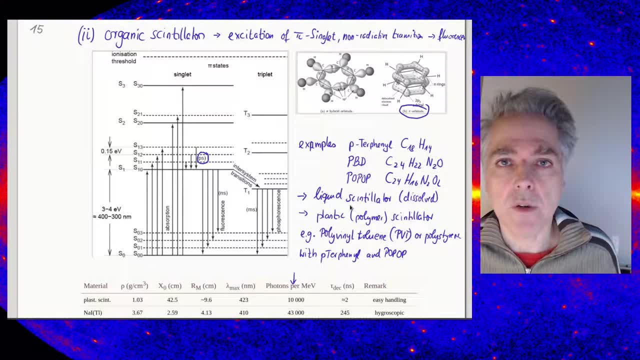 a scintillator material and that is then usually dissolved in the form of a liquid scintillator or added to some polymer to form some plastic which you can then form and you can use it in any kind of shape you want. Here's a big table which basically lists some 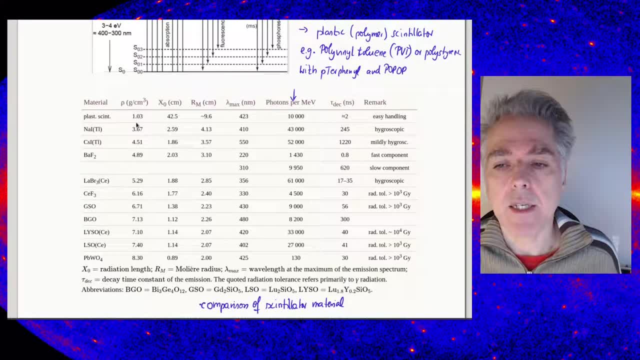 of the main properties of the scintillating material. So, as I said originally, the density is much smaller than for organic, than for inorganic. For inorganic there's, for example, sodium iodine, which has a doping with tellurium to increase the efficiency, or cesium iodine. 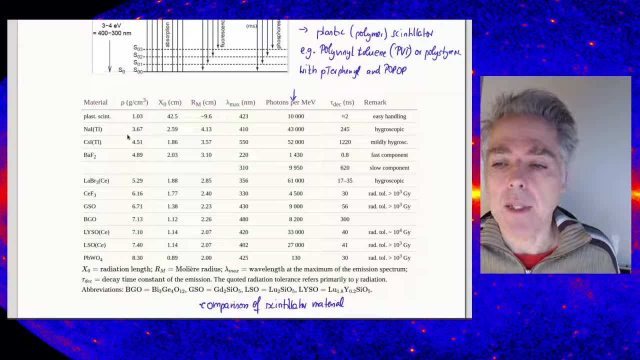 with tellurium doping also a similar way, And these are the most common scintillator materials which are used. Sodium iodine has the disadvantage that it's very hygroscopic, so you have to sheet it from water, otherwise it basically dissolves. 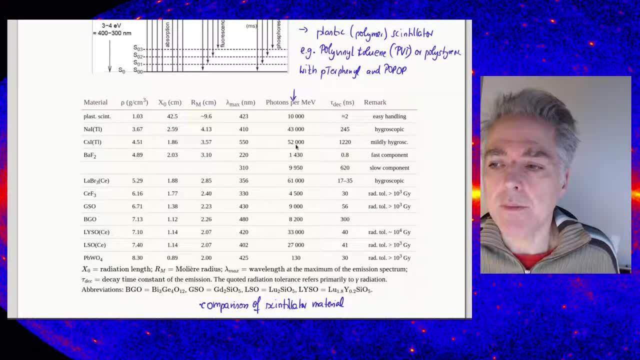 And cesium iodine is, together with sodium iodine, really the most effective one. That is, you produce something like 50,000 photons per MeV energy deposited, which is quite substantial. However, the time scale of these transitions taking place is of the order of hundreds of. 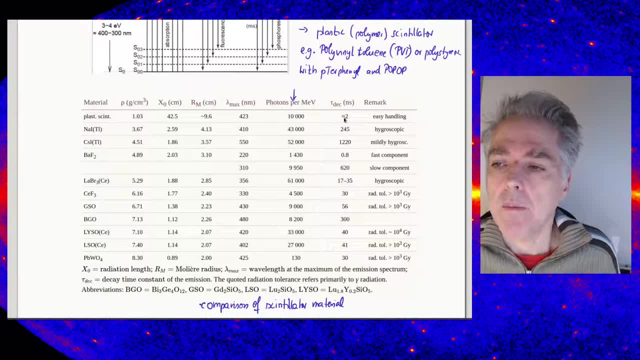 nanoseconds, so this is rather slow. This is different for the de-excitation in plastic scintillator materials And here's some additional crystal-type samples which I used, which, however, share some advantages and disadvantages which relate to the material properties. It could be very brittle, very 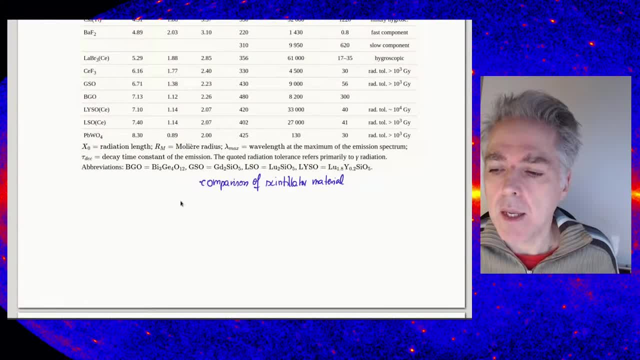 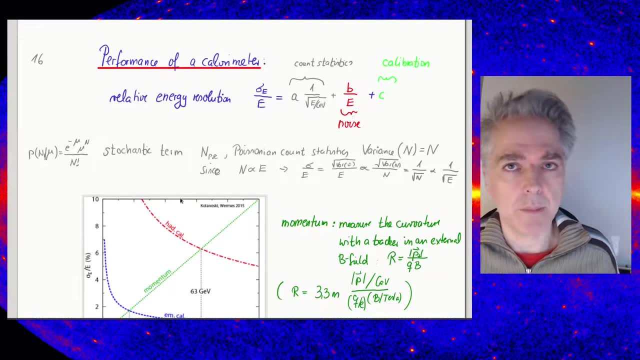 hygroscopic, and so on and so forth. Now let's look at the performance of a calorimeter once more, because I discussed a little bit now what a calorimeter could be made of- so like a sandwich sampling type calorimeter- And what is, however, the energy resolution that we can push these calorimeters Again. 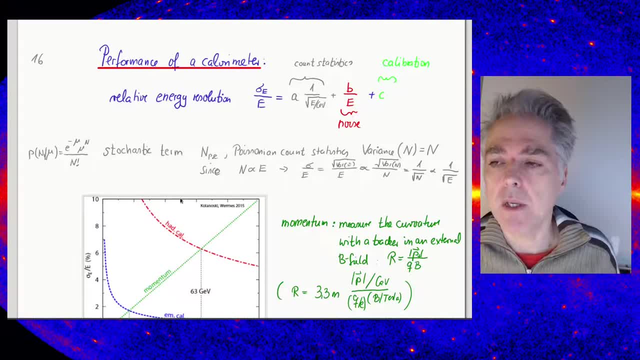 I just make the discussion mainly for the electromagnetic calorimeter. So the relative energy resolution, sigma e over e, depends upon a number of issues. So let's talk about for a moment what a calorimeter does. again, It counts number of particles, So on average, 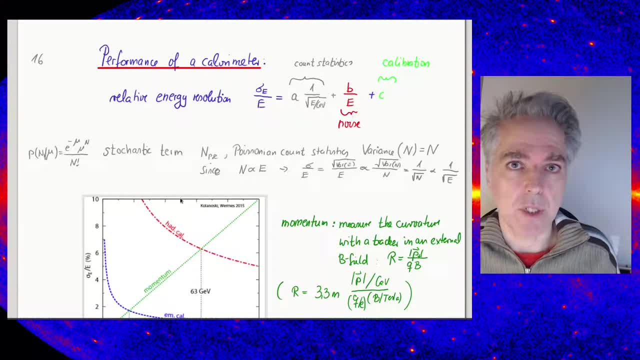 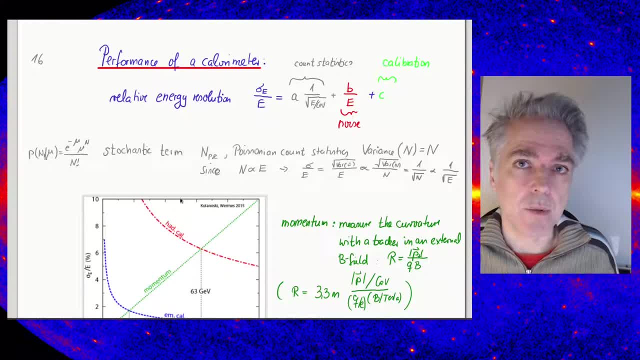 particles produced in such a secondary cascade And you count them all. Let's say with a hundred particles produced in such a secondary cascade And you count them all. Let's say with a hundred is essentially the Poissonian count statistics, And I give the probability density function here. 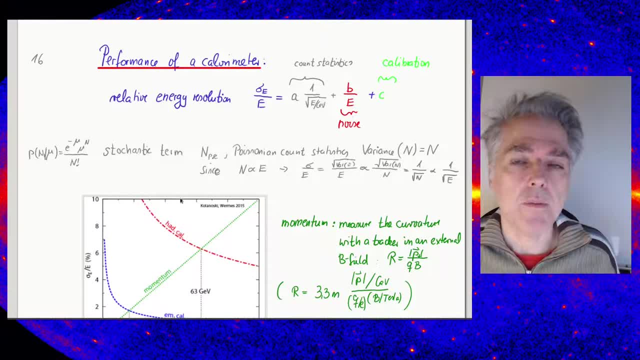 So for some expectation value mu, you would have a probability to count n particles, which is given by this exponential to the minus mu times mu, to the power of n divided by n for quartet. This is something which is stochastic you cannot avoid. 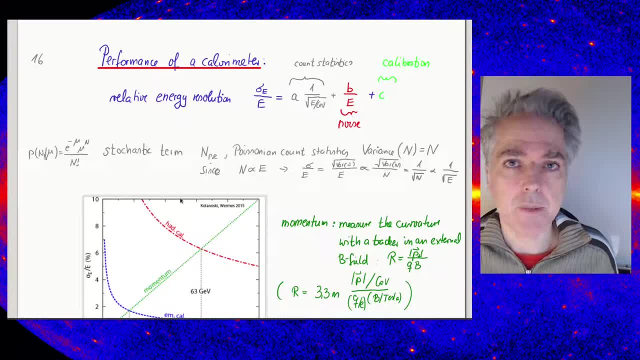 So the only thing you can make, you can improve this by having more particles. but again, this is energy dependent. You cannot just create new particles out of thin air. They have to be coming from the initial energy. So the number of particles that you will measure will fluctuate. 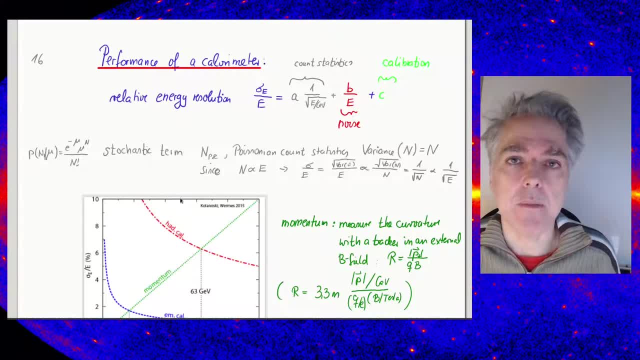 And for the Poissonian statistics, the fluctuation or the variance of that number is given by its expectation value. So expectation value, if you measure something, is, in the simple interpretation, simply the number of particles you measure. So the variance of this number is then given by the number itself. 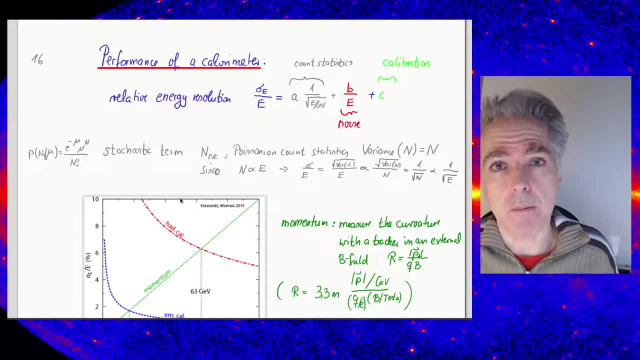 So let's assume you have 100 particles which you detect, Then you know that the variance of that number is 100.. The square root of the variance gives you then how a measure of the width of your distribution that you would measure. 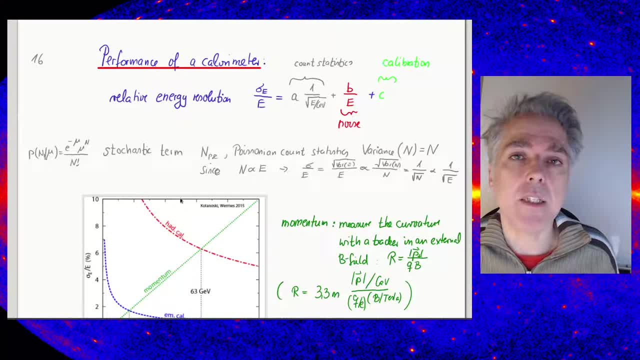 is then 10.. So you would measure roughly 100 particles plus minus 10. That would be a 10% energy resolution. If you go for 10,000 particles, then you would have a variance of 10,000, square root of that is 100.. 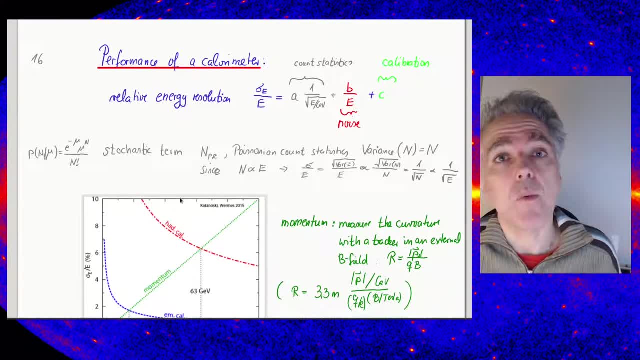 So that means that, basically, you would measure 1% relative uncertainty of your energy. So you see, the uncertainty gets smaller, the relative uncertainty gets smaller and smaller and smaller, and does that with 1 over the square root of the energy. So this is then the first term which you usually have to consider. 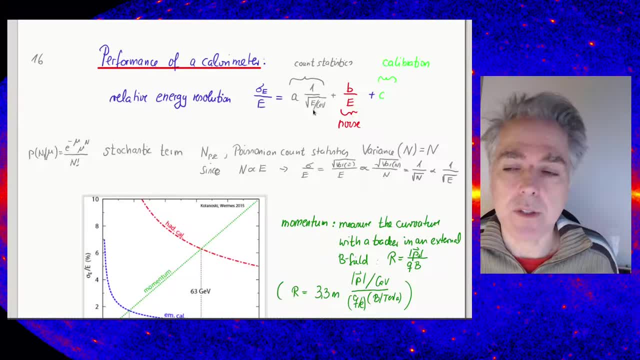 because this is something which you cannot get around with the count statistics term here, So that all goes with 1 over square root e, And I just introduce here a pre-factor a, because you have some efficiency losses and you have to take some 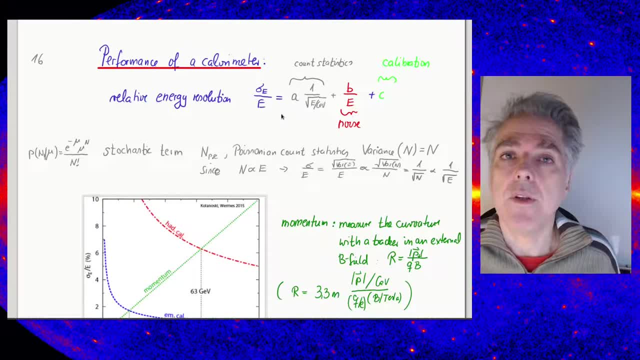 conversion into account, and so on and so forth. Now there's a second thing which happens, that is, basically your number of particles that you measure will also fluctuate, given that you have some particles which you lose, you have some particles which may not convert. 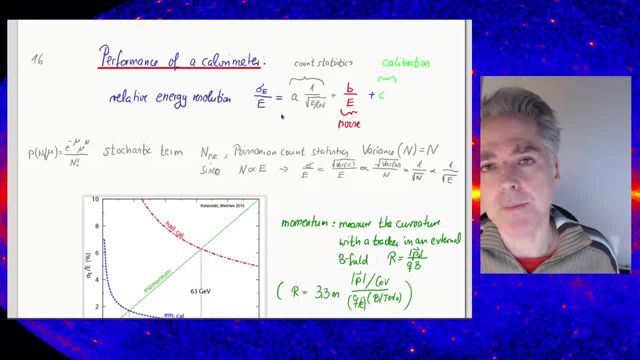 because of efficiency issues and so on and so forth. So you have some intrinsic uncertainty, And that is constant. So you will always measure some. let's say you will always measure something like 10 particles deviation. So it could be that, on top of the Poissonian fluctuation, 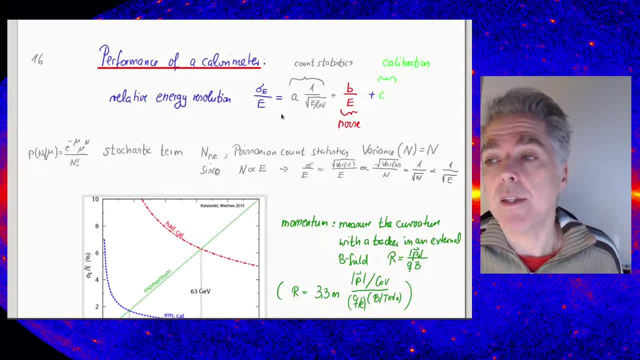 you have always some additional uncertainty, And that is then this B term- here I call this the noise term- And that will be dominating at low energies, because this goes with B over e, because this is simply a constant sigma term, which is energy independent. 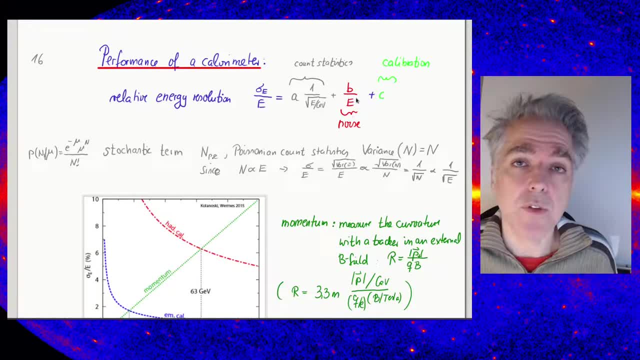 and the relative uncertainty goes with B over e. So for small values of e, this will always be the dominating performant term, And whereas then, at higher and higher energies, you will be dominated by this count statistics term. there is another thing which happens. 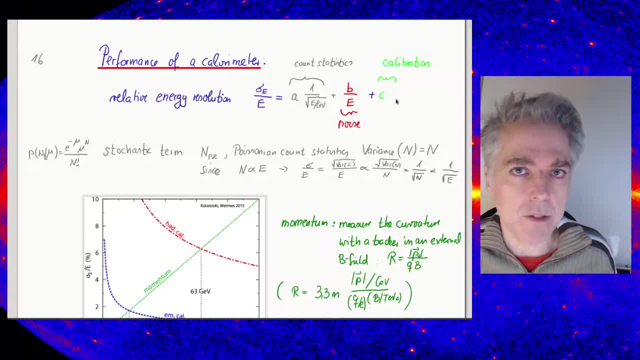 that is, you will have some calibration, some generic uncertainties which come into the game from your setup and they are actually giving you a relative uncertainty which is constant, So let's say like a 1% uncertainty which you will always have, And this will eventually dominate at the highest energies. 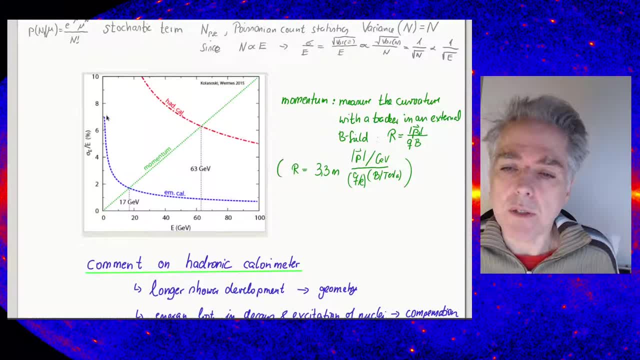 because it is constant. So for typical values, let's say a very well performing electromagnetic calorimeter, you will basically see that the energy resolution- now this is plotted here as a function of energy- goes down. so the lower part, it goes with 1 over e.